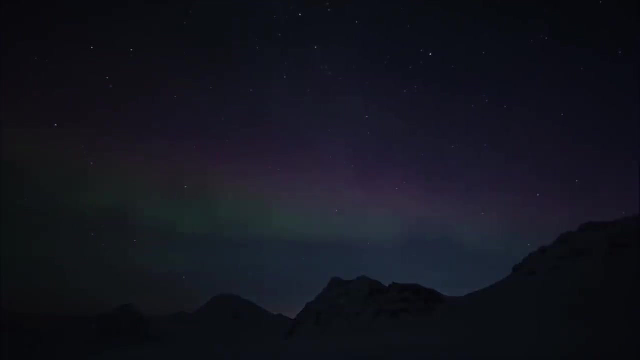 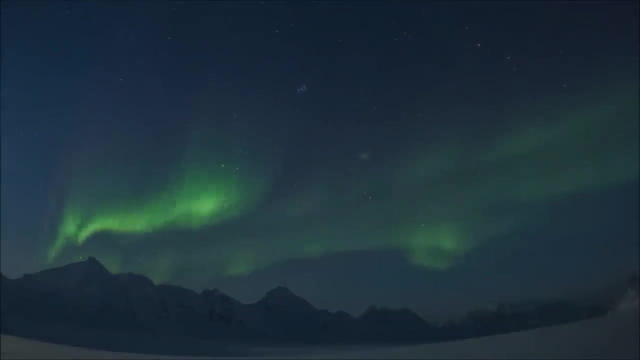 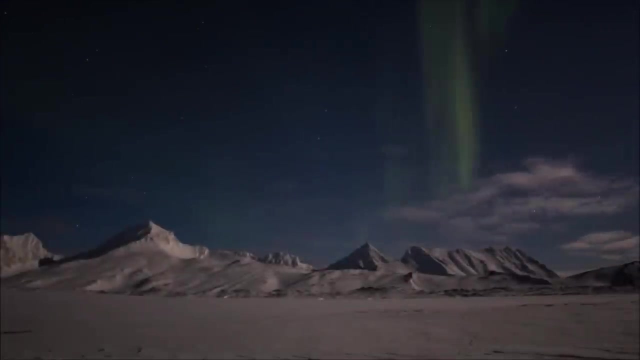 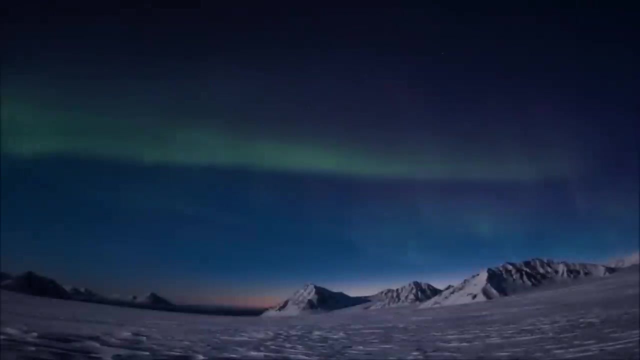 They have fascinated people for thousands of years. Some people once thought they were spirits dancing in the sky. Others thought they were the flames of dragons. Today's scientists have learned that the auroras are caused by charged particles from the sun that interact with the Earth's magnetosphere, exciting the gases of the atmosphere until 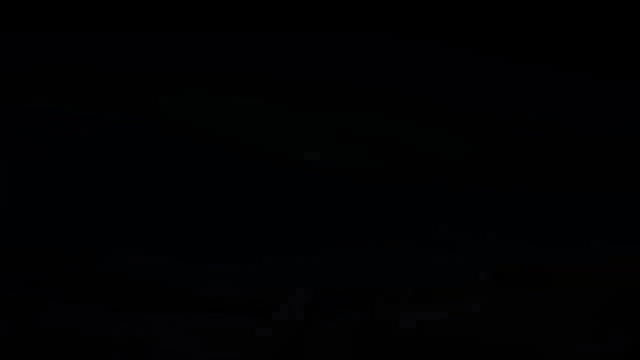 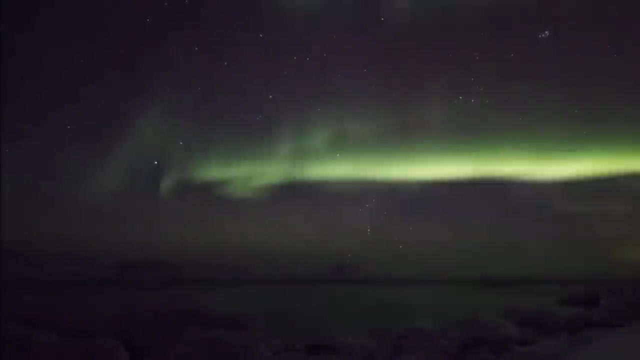 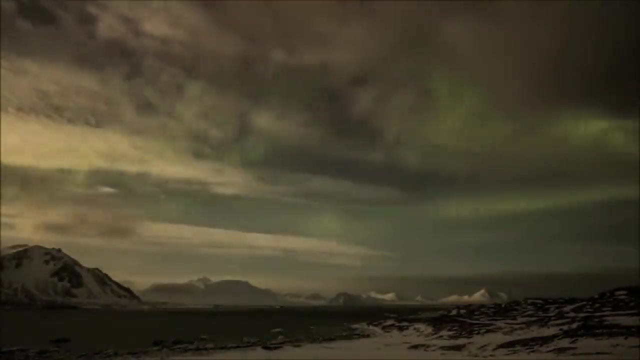 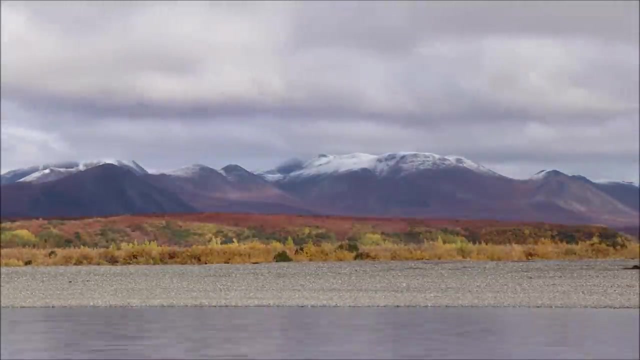 it glows. The auroras will also occur in the skies surrounding the South Pole, where they are called the Southern Lights. Any place on Earth far enough north that it has at least one night where the sun does not set and one day where the sun does not rise is considered to be inside the arctic. 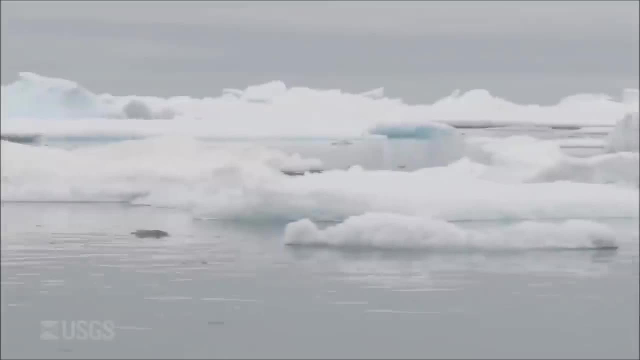 circle. The Arctic Circle is an imaginary line that encircles the North Pole at about 60 km per second And if you try twelve times it will crash into your l Team 2 rocket and74, our C Front link flightissant Grant, shewisham S22 and almost 40 seconds back. 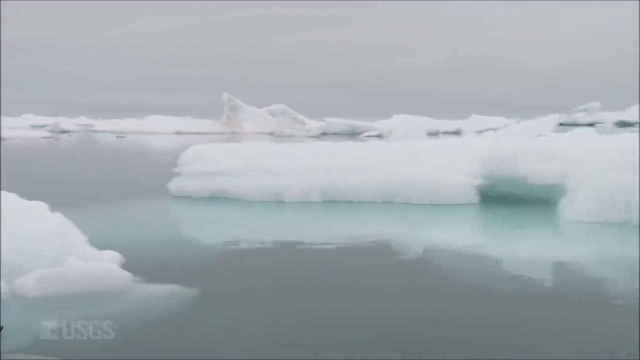 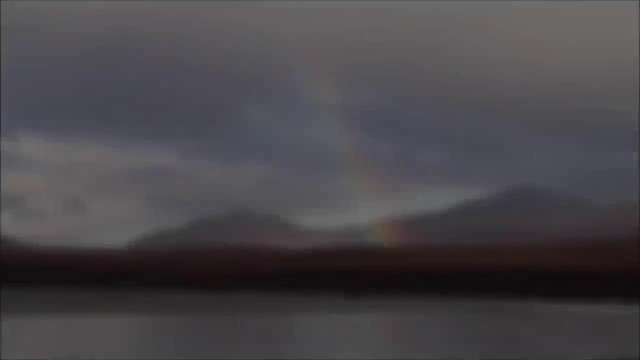 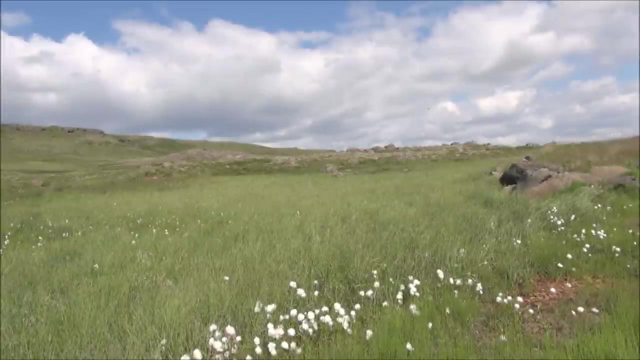 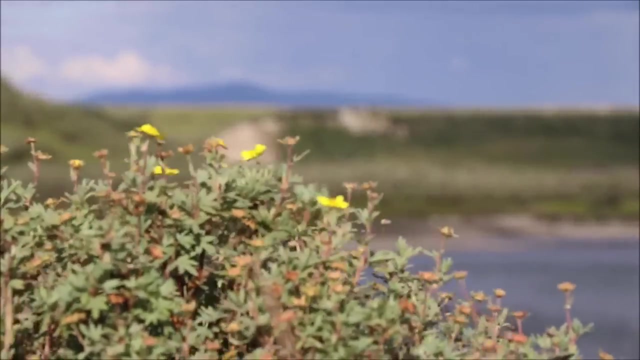 Borealis may occur on выз forforth 66 degrees north latitude. The Arctic is mostly ocean, but it also includes parts of Greenland, Canada, the United States, Russia, Norway, Finland, Sweden and Iceland. Lands at the southern edges of the Arctic Circle are generally covered by tundra. 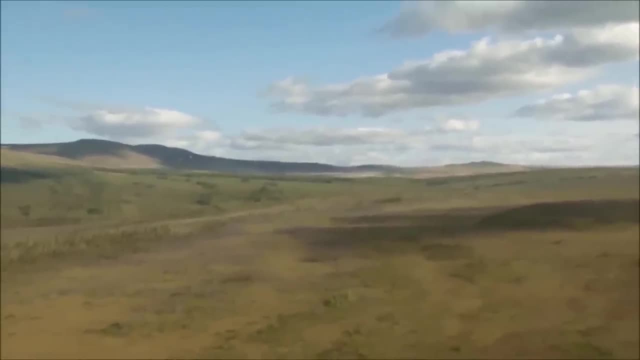 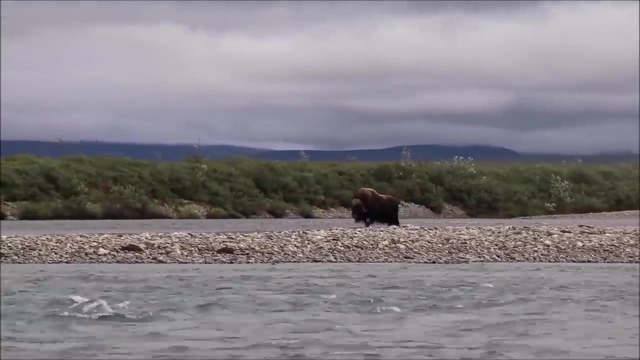 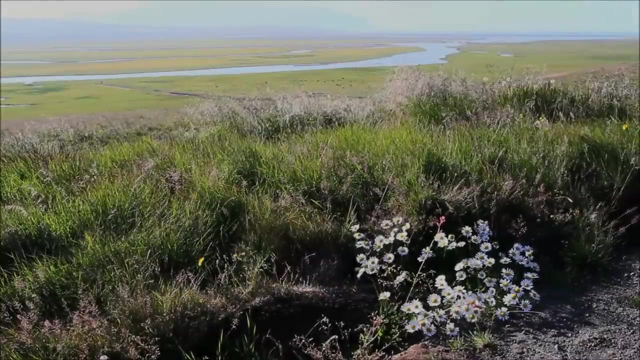 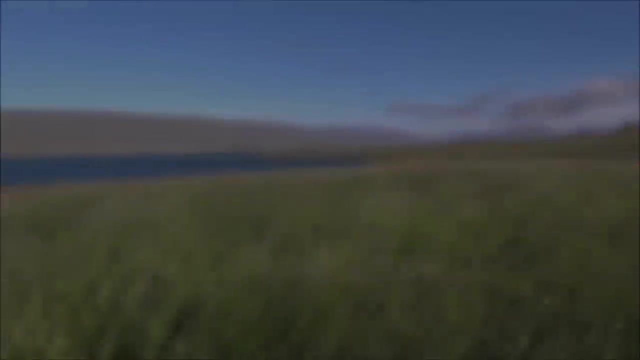 The tundra is vast and for the most part treeless. The short Arctic summers are too cool and too brief to allow trees to flourish here. But there is another barrier as well – permafrost Beneath a thin active layer of soil that thaws and refreezes every year the ground. 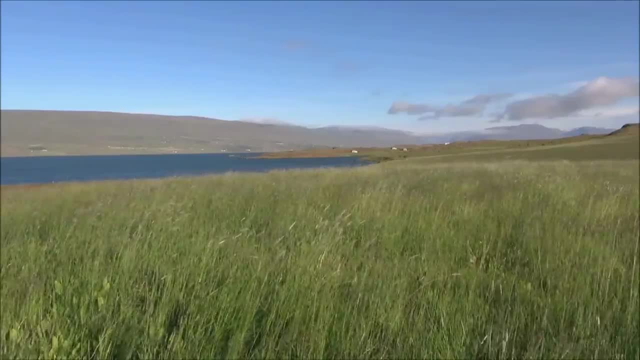 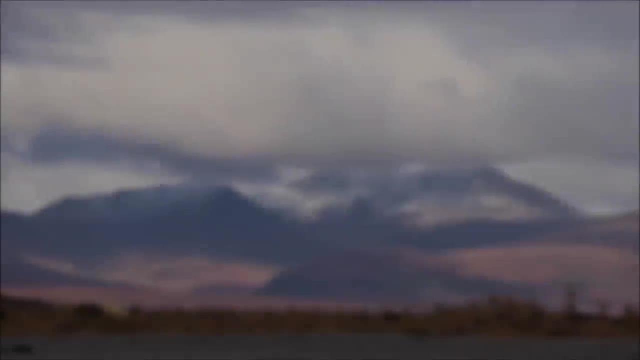 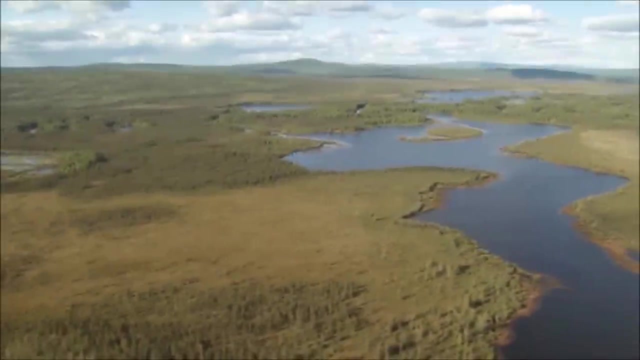 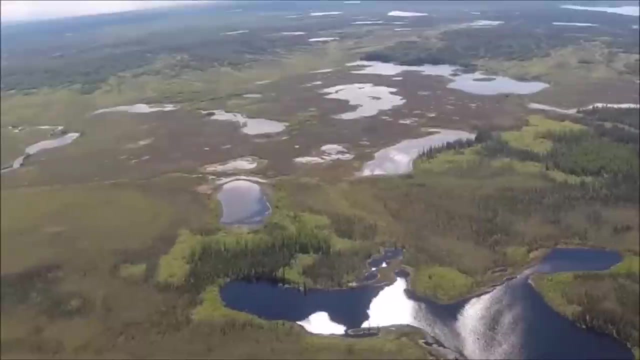 is permanently frozen, The plants that survive…. …mostly grass, moss and shrubs, grow close to the ground and have shallow roots. Although there is little rain on the tundra, summer is very wet. The frozen upper layer of soil thaws out, but water cannot sink into the ground past. the frozen barrier of the permafrost. Since temperatures there rarely climb higher than 54 degrees Celsius, the permafrost is very cold. If the temperature is higher than 54 degrees Fahrenheit or 12 degrees Celsius, very little of the water evaporates. 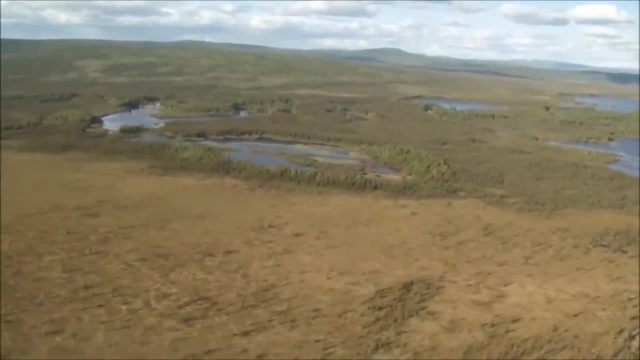 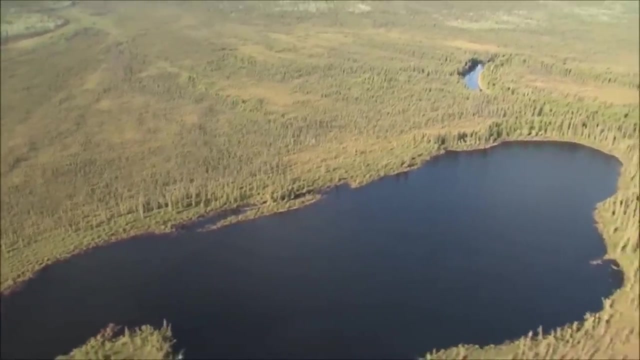 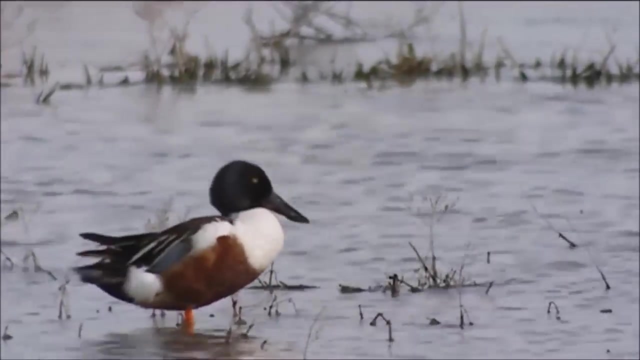 Instead, it sits on top of the permafrost layer, forming lakes and marshes that will turn to ice as soon as temperatures sink below freezing once more. Many birds, especially waterfowl, will migrate north to these cool summer wetlands in the 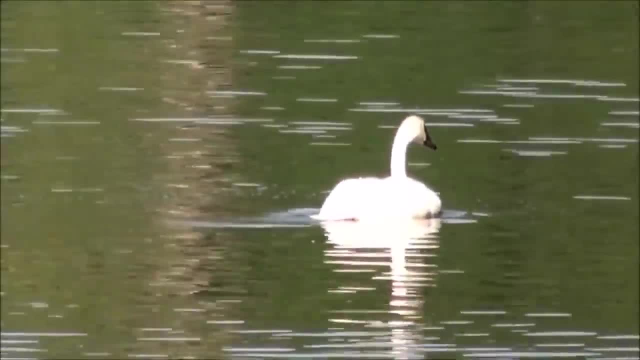 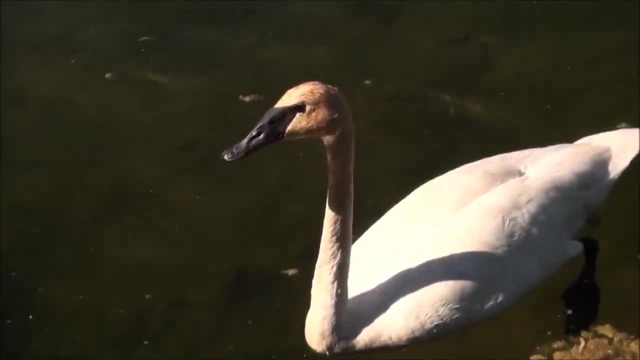 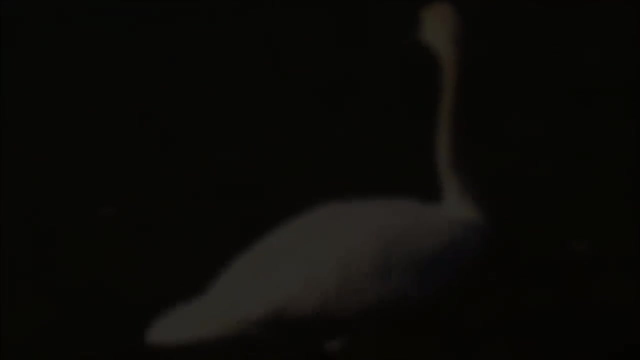 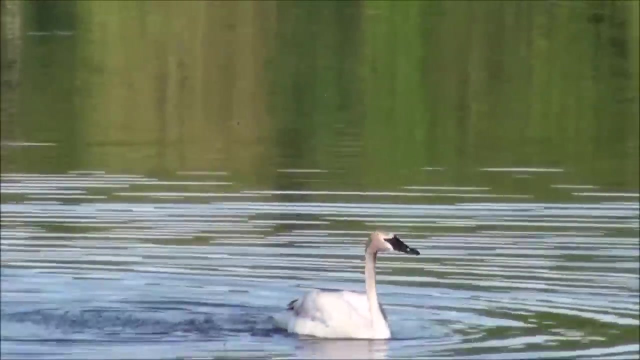 Arctic. One bird that does this is the trumpeter swan, with some flying from wintering grounds as far south as Texas or Mexico, With adults frequently reaching weights of 30 pounds or 13.6 kilograms. it is the heaviest bird living that is native to North America. 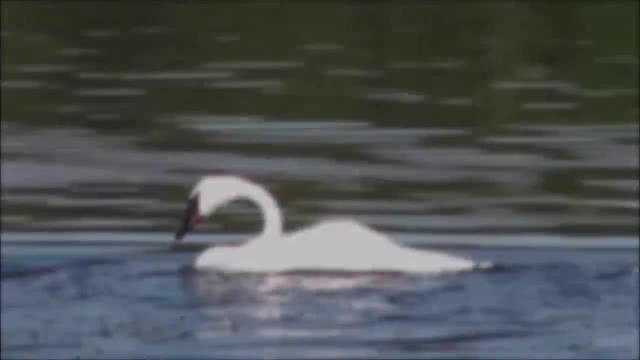 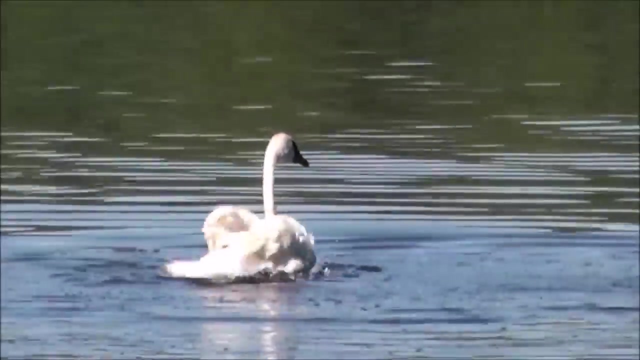 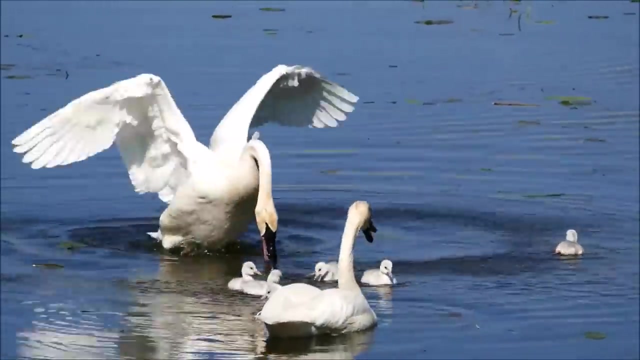 It is also the largest species of waterfowl. It is the largest species of waterfowl in the world, with a wingspan that can surpass 10 feet or 3 meters. The Arctic wetlands provide an important habitat for the trumpeter swan, a refuge from hunters. 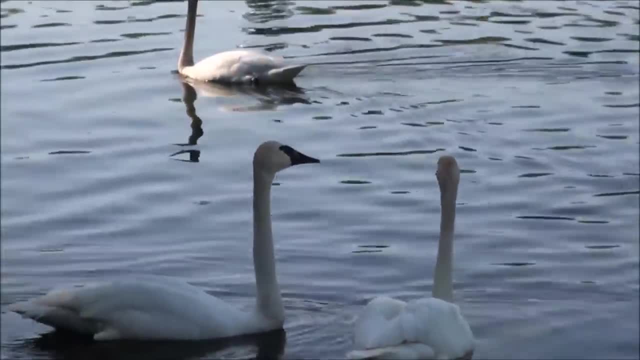 that decimated populations in Canada and the northern United States near the beginning of the 20th century. By 1933, only a few dozen of them would survive. The trumpeter swan is the largest species of waterfowl in the world, with a wingspan that. 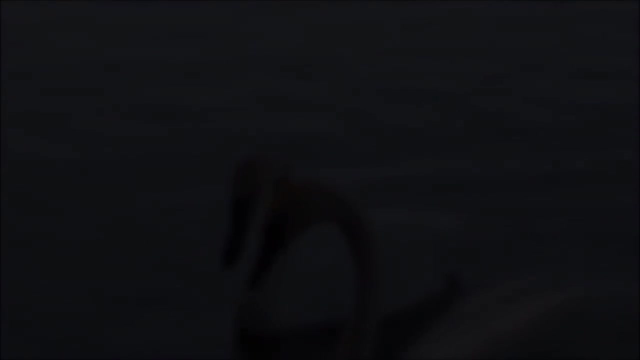 can surpass 10 feet or 3 meters. The Arctic wetlands provide an important habitat for the trumpeter swan, a refuge from hunters that decimated populations in Canada and the northern United States. near the beginning of the 20th century, Only a few dozen wild trumpeters could be found in these southern areas and people feared. 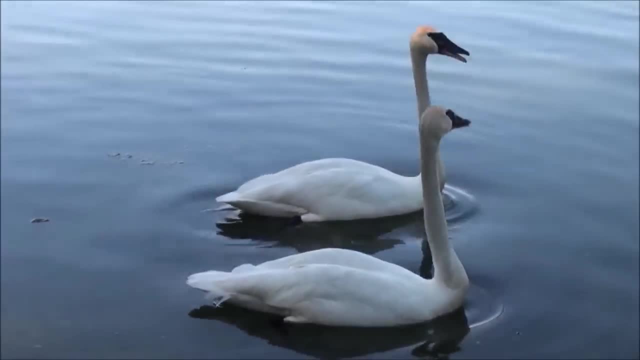 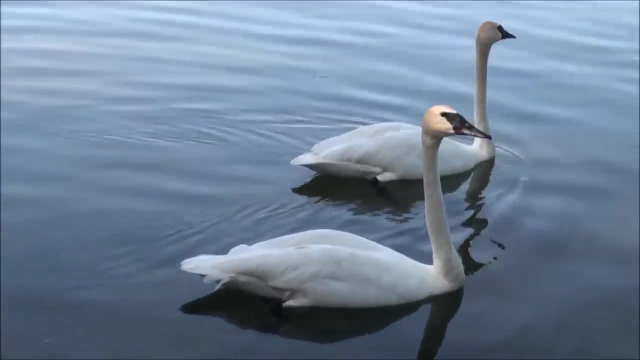 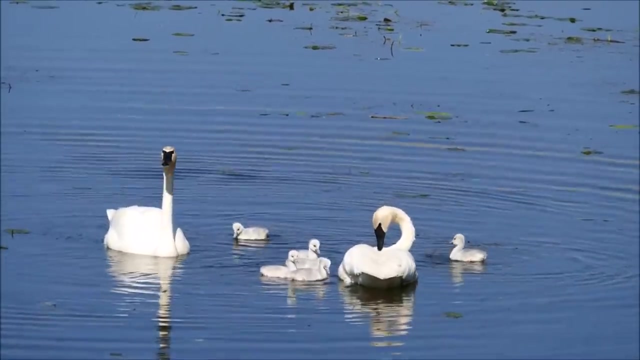 they would become extinct. Then a second population of trumpeter swans was discovered up in Alaska. thousands of them- Some of the Alaskan swans- were carefully introduced to the areas where trumpeters had been overhunted, allowing the populations to recover. 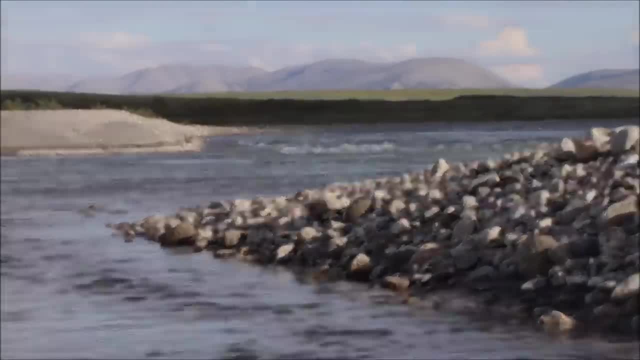 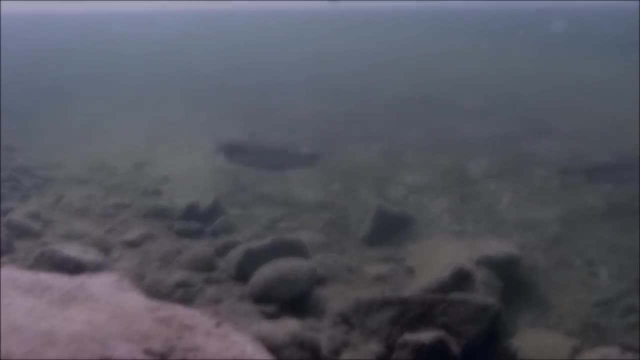 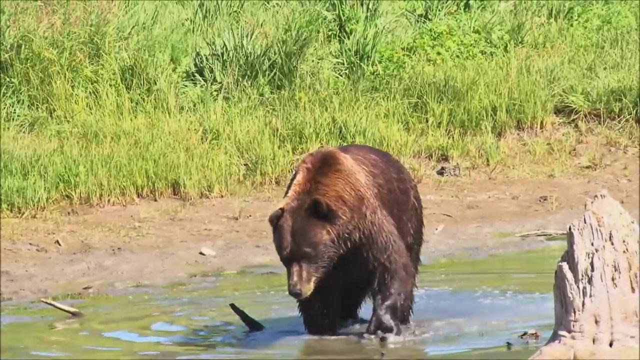 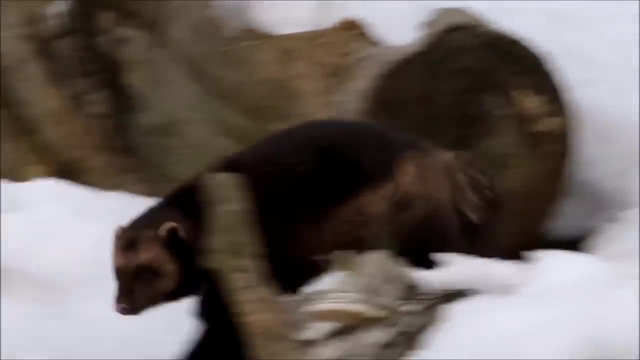 Waterfowl are not the only animals to make their home on the tundra. Fish like salmon and cod migrate to the waterways there each year. The fish in turn attract predators like bear and eagles. Wolverine and fox live here too, as well as musk, ox and caribou. 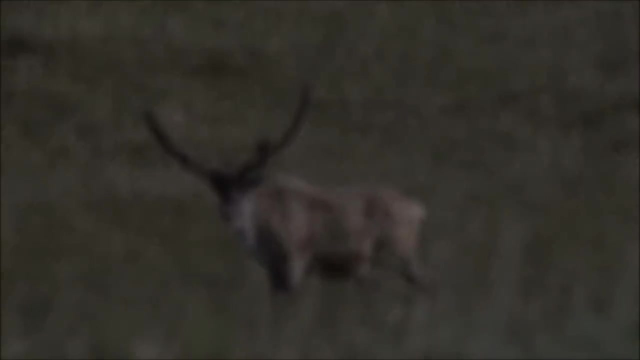 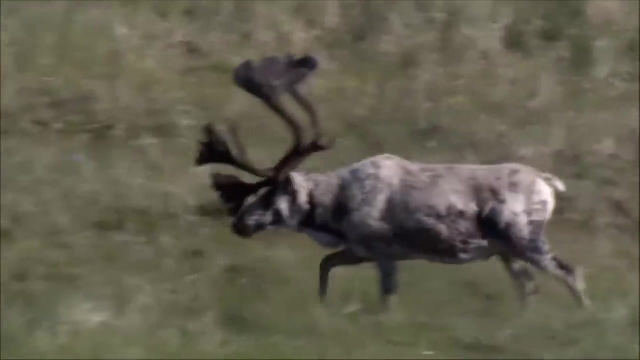 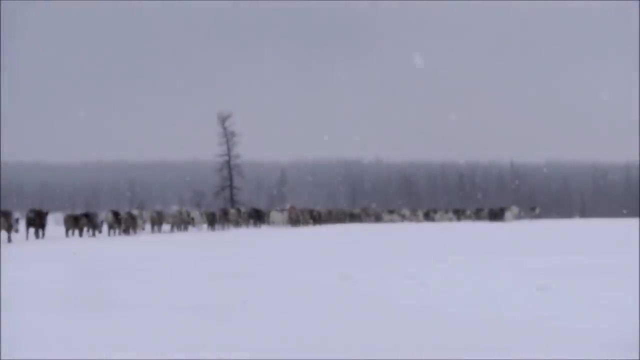 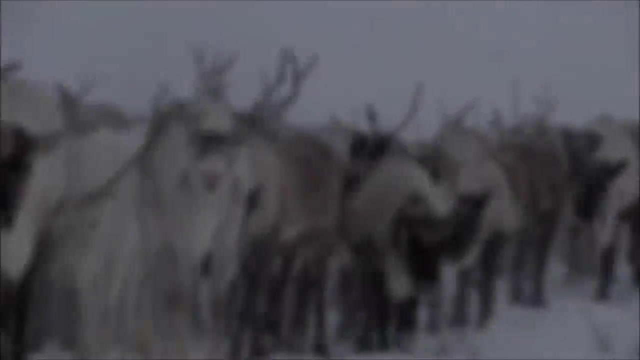 Caribou or reindeer, are one of the world's great migrators. In the winter they travel south to snowy pine forests. They cannot survive farther north where the snow is too deep, because they must dig through the snow to eat the moss and lichens beneath it. In the spring, they migrate north again to take advantage of the plants that are growing in the water. They can also eat the moss and lichens beneath it. In the spring, they migrate north again to take advantage of the plants that are growing. 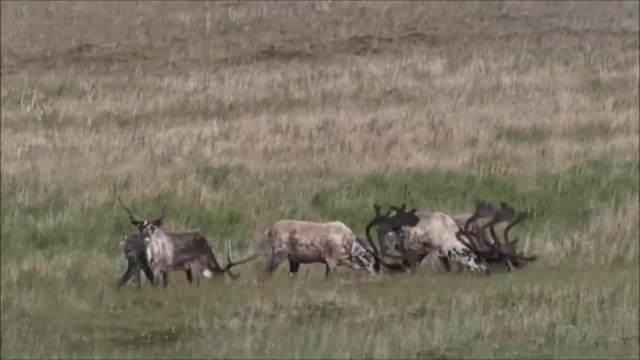 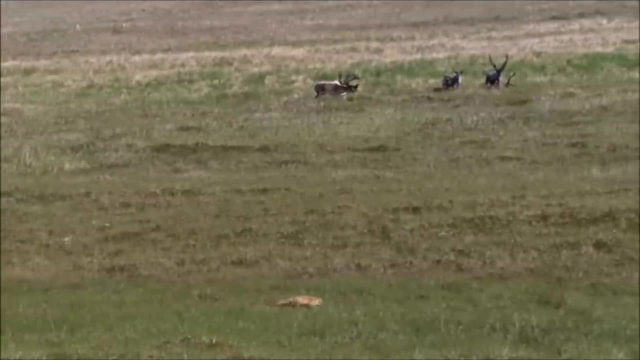 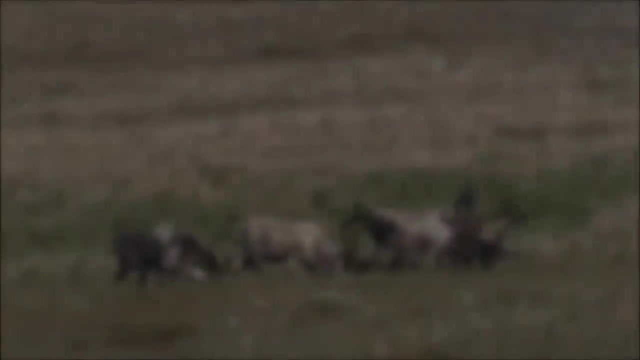 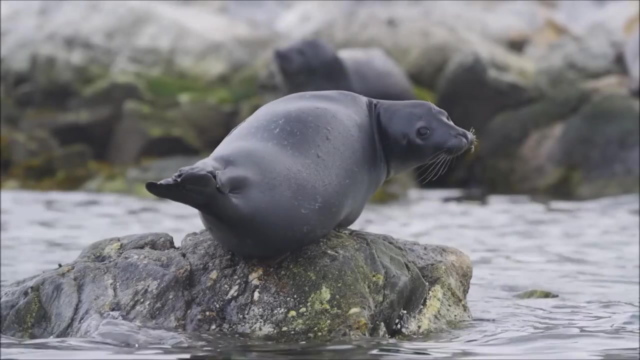 on the tundra and birth their calves. Some North American caribou have the longest migration of any land mammal in the world – up to 3,000 miles or 5,000 kilometers. Animals attempting to survive in the Arctic need every advantage they can get, and some 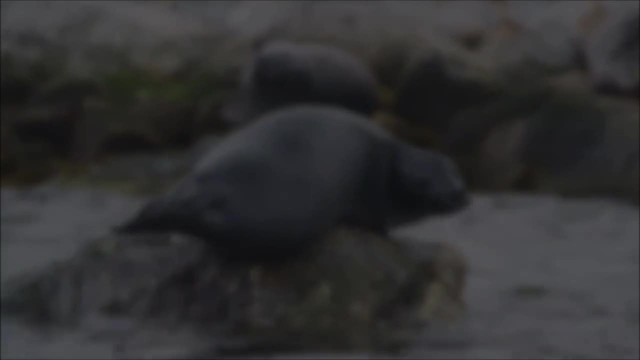 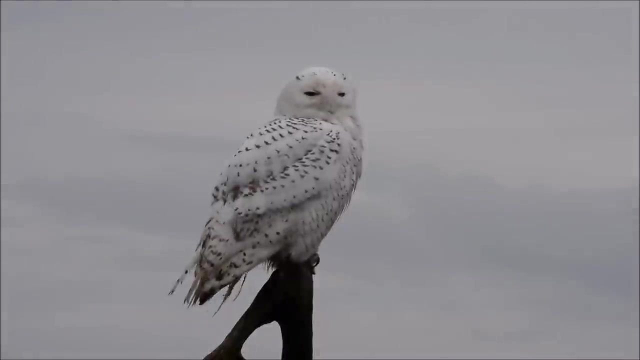 have found it by changing their appearance. In a land of ice and snow, it is sometimes helpful to be white yourself. Some animals, like the snowy owl, keep white feathers year round. Others, like the arctic fox, wear brown or grey fur in the summer and only turn white. 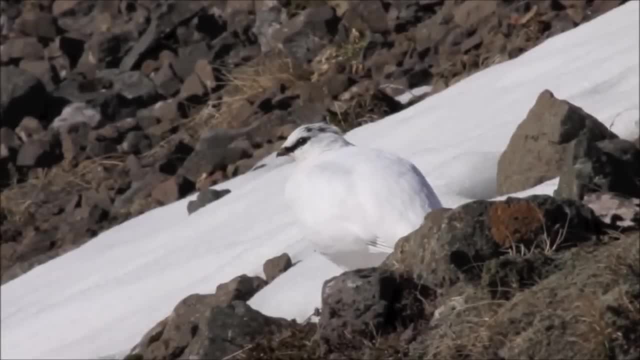 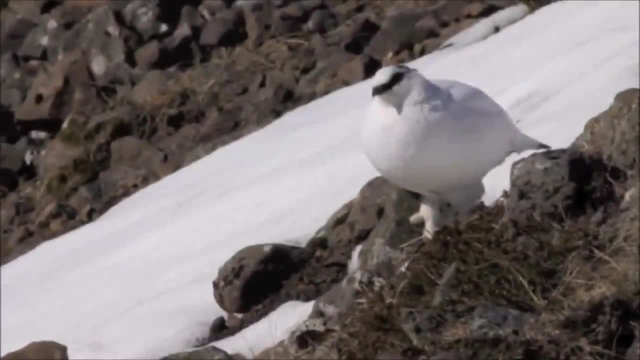 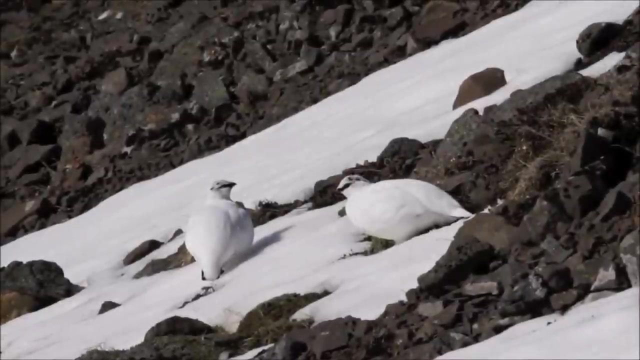 in the winter. Another color changer is the ptarmigan, Covered in patchy brown and white feathers. in the summer, they begin to change their plumage as the days shorten. Both male and female ptarmigans will go through the winter in a coat of nearly pure white. 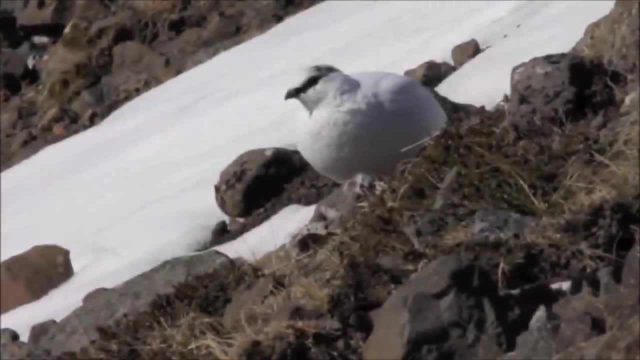 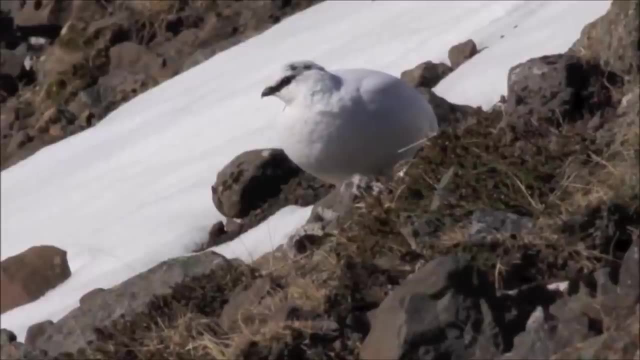 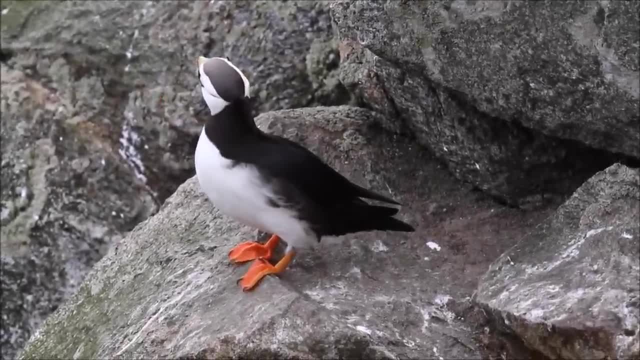 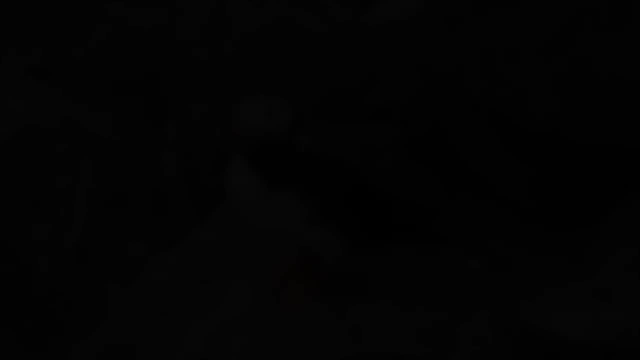 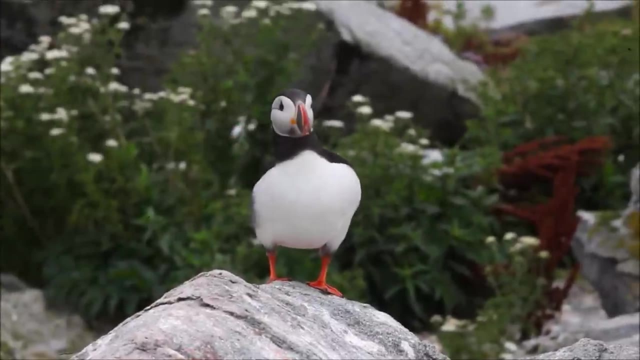 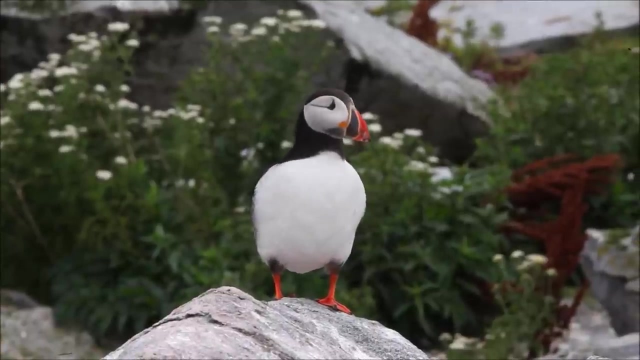 Puffins are seabirds. They only return to land to breed, nesting in burrows dug in clifftops. They prefer to breed on islands where risk from land predators is much lower. Puffins spend months at a time out on the open ocean, and it is out at sea that their coloring 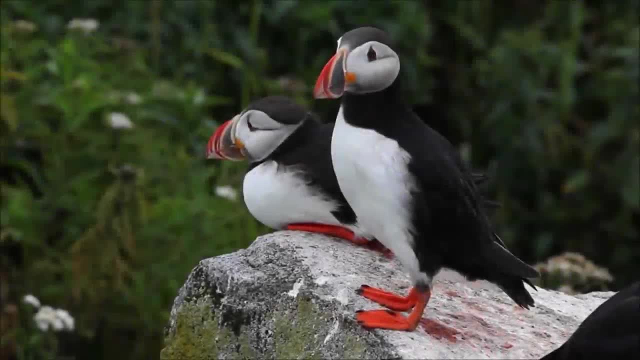 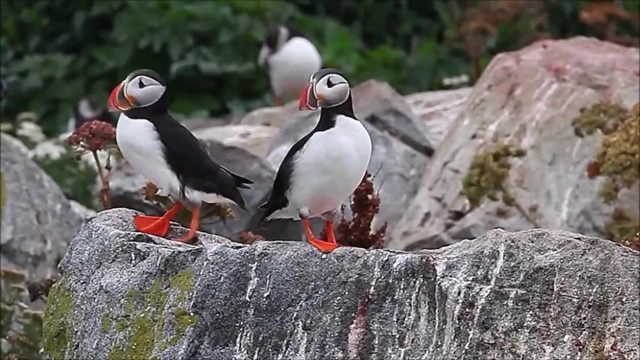 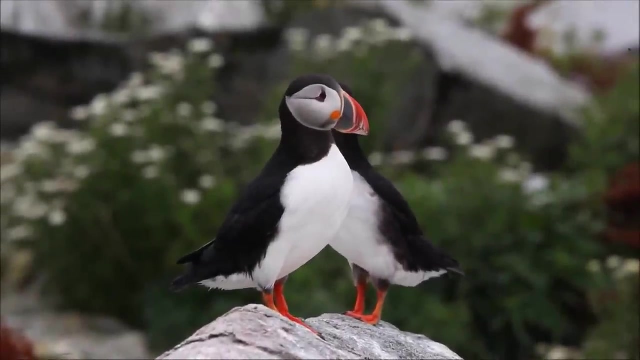 comes in handy. They have black feathers on their backs and white feathers on their stomachs. This color pattern is called countershading, and it helps them blend in to the dark ocean water when seen from above or the bright sky when seen from below. 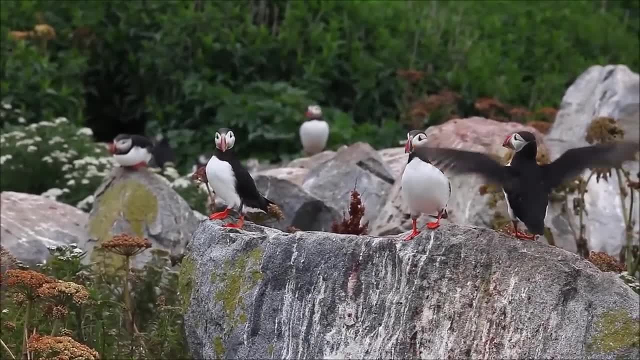 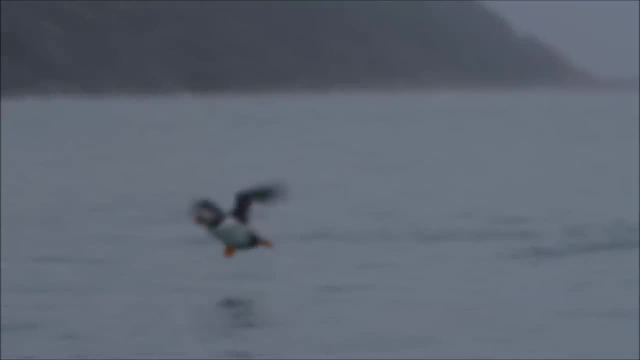 Although they can fly, puffins are awkward in the air and typically move around by paddling their webbed feet. as they sit on the water's surface To catch fish, they dive, moving along by flapping their wings underwater, much as penguins. 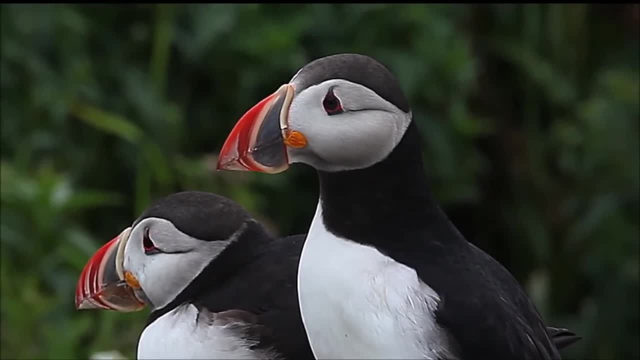 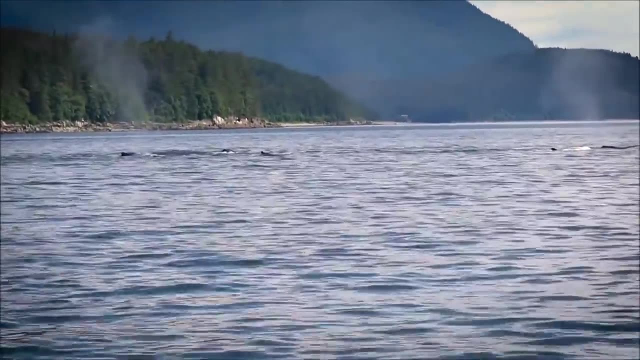 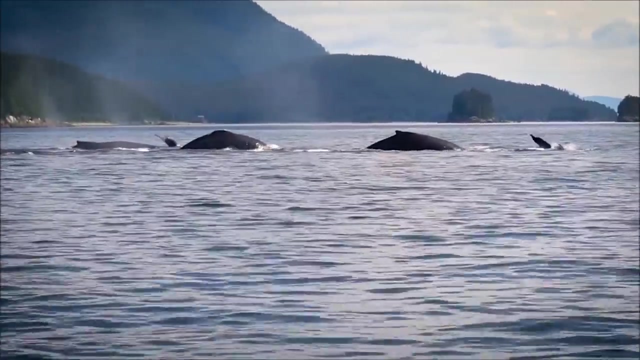 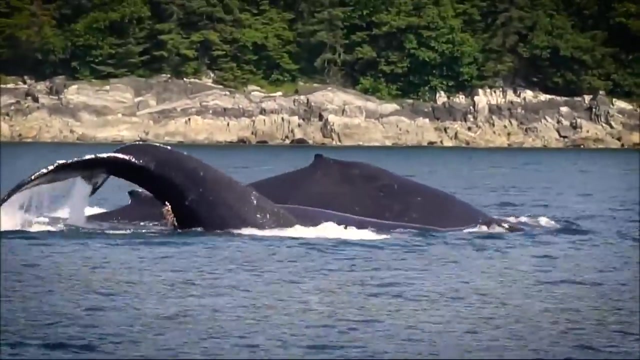 do. The rich feeding grounds of the northern oceans attract larger animals than puffins – much larger Humpback whales travel north in the spring to feed on the krill and small fish abundant in the frigid waters. Although humpbacks are often solitary, they sometimes form small groups, especially when 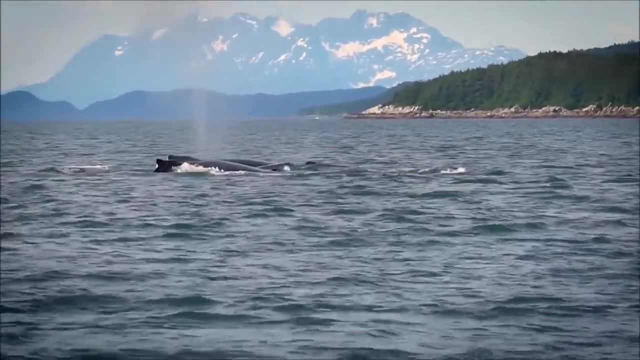 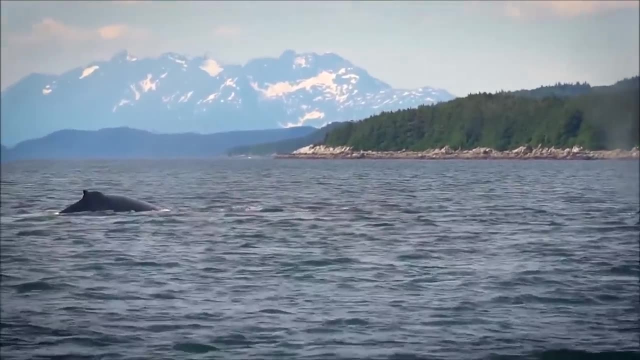 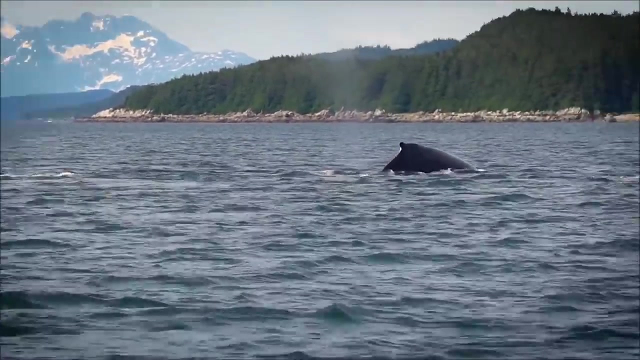 hunting. A group of humpback whales together can use a special method called bubble netting to trap fish and krill. The whales will surround and circle a school of fish. 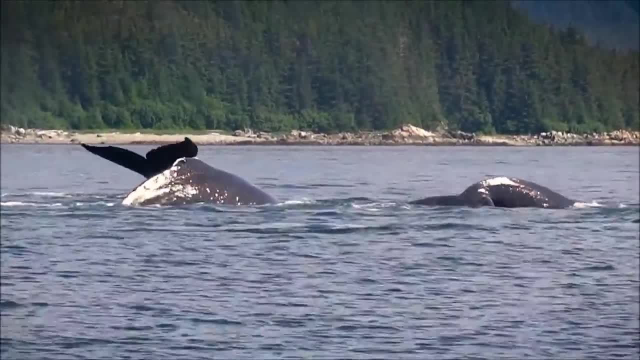 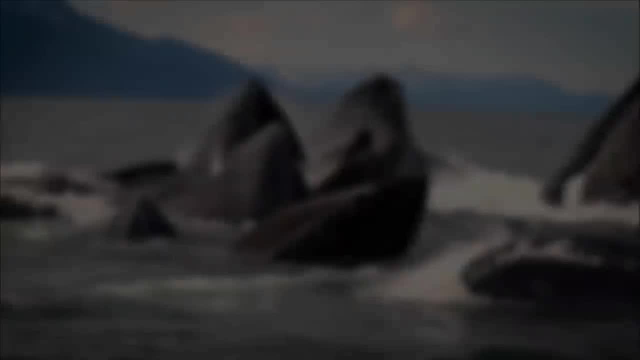 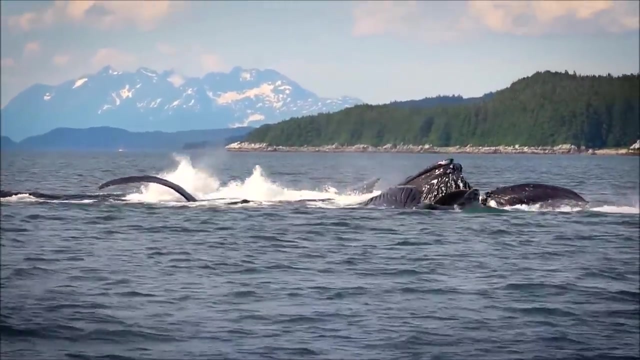 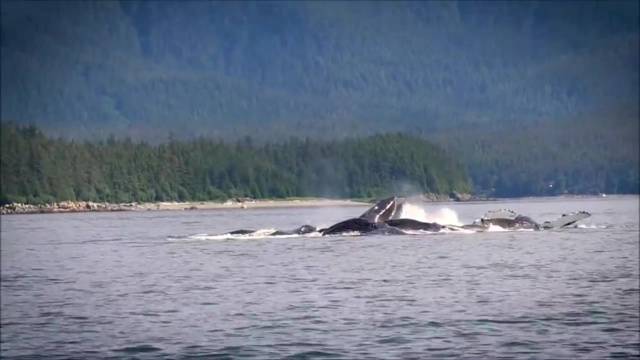 Then other whales begin blowing a ring of bubbles to trap them. Once the fish are trapped close together, the whales will come up from beneath them mouths wide open, scooping up huge quantities of fish like a net. Their baleen plates allow them to strain the tiny creatures from the seawater. 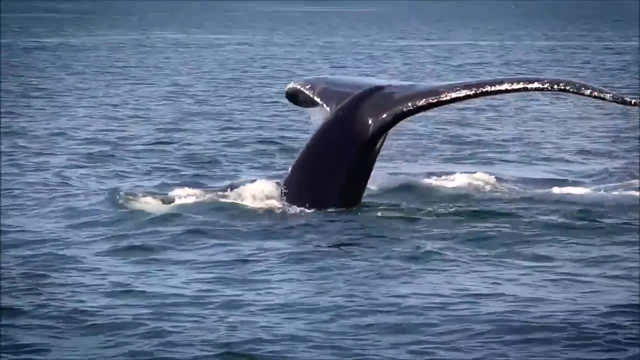 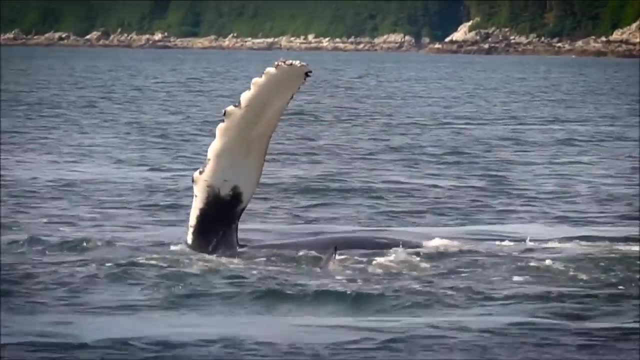 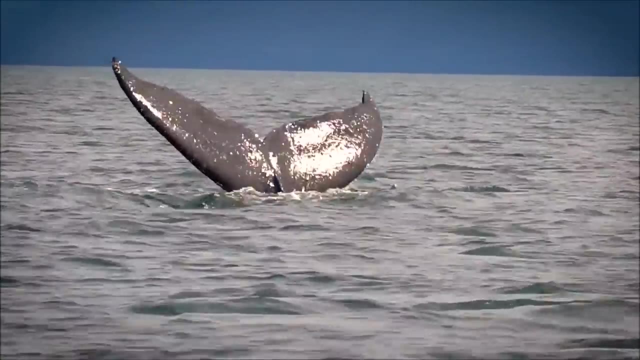 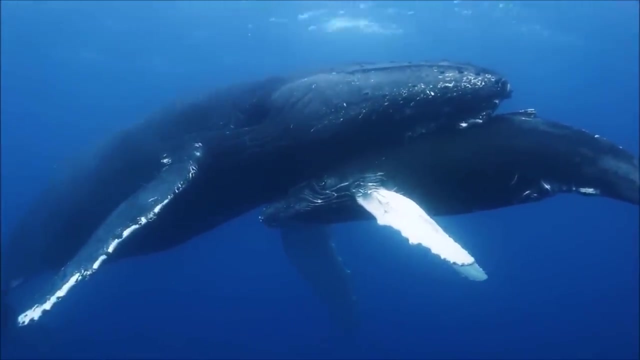 The humpbacks must eat massive amounts of food in the spring and summer months to build up their fat stores. When the weather turns cold, they will migrate to warmer tropical waters and they will not eat again until the spring. It is in these warmer waters that they mate and give birth. 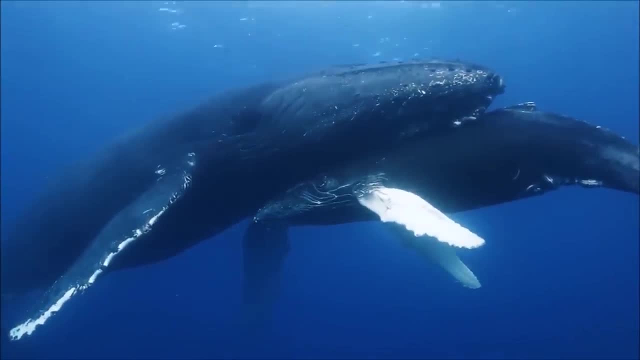 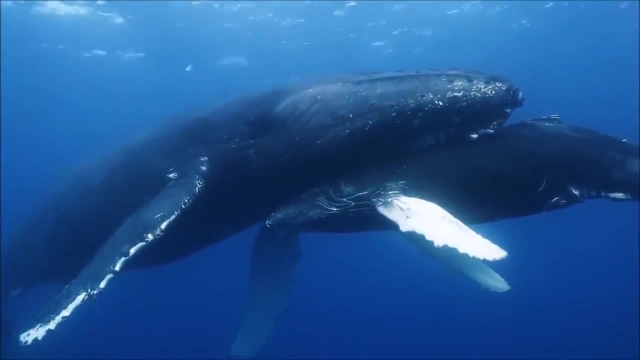 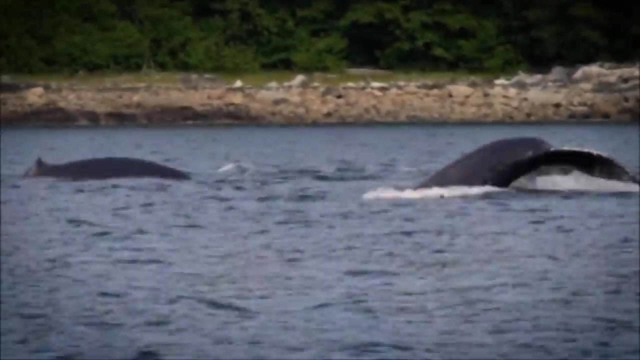 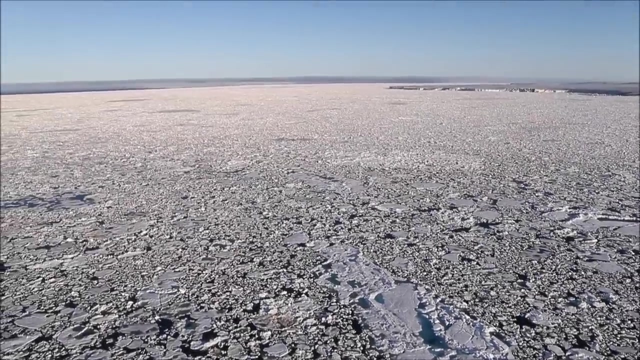 Newborn calves could not survive the freezing temperatures near the poles. It is important for the adults to have successful summer hunts so that they can survive their yearly migration. As we travel farther north, we come to areas where the snow and ice never completely melt. 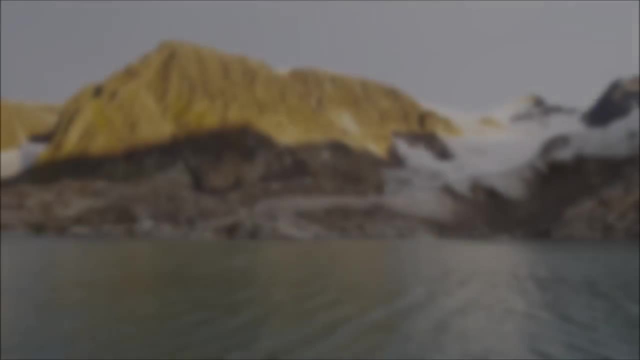 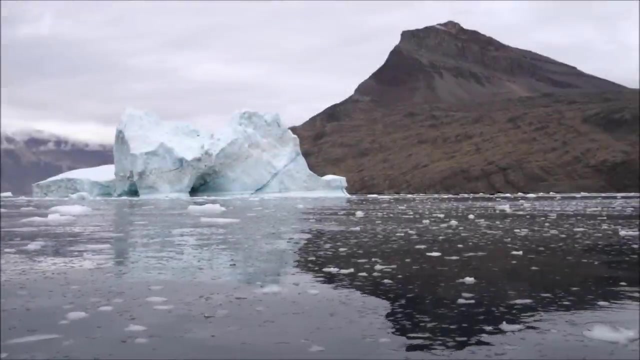 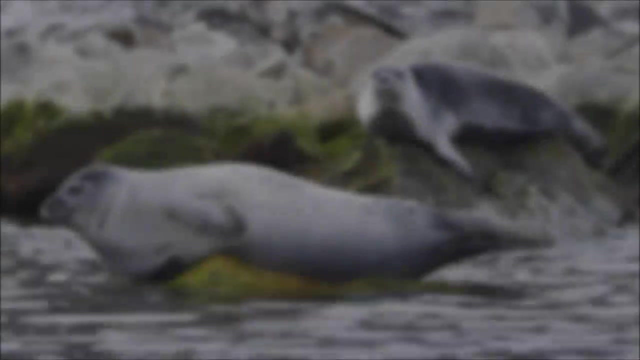 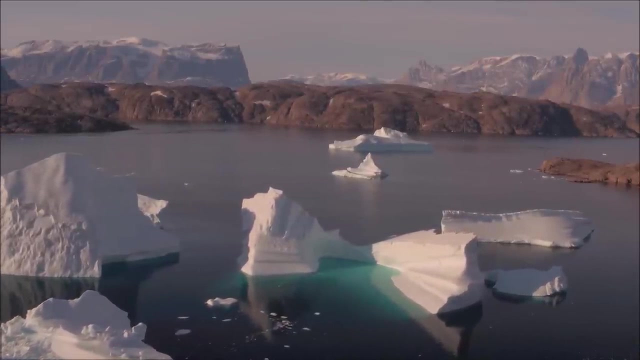 – and the ice is never completely melted In a place called the High Arctic. Even here there is life. Instead of tundra, the High Arctic has polar barrens. Far fewer plants survive here, mainly moss and lichens. As a result, most food chains do not rely on land-growing plants. 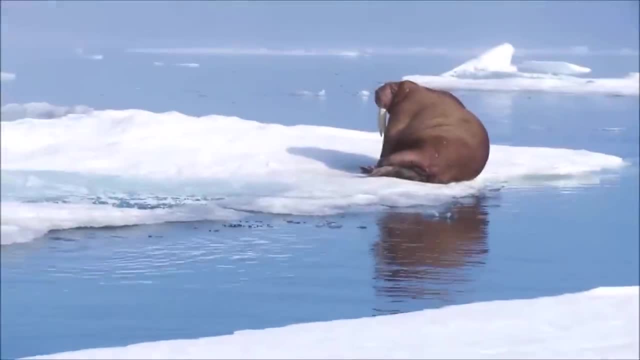 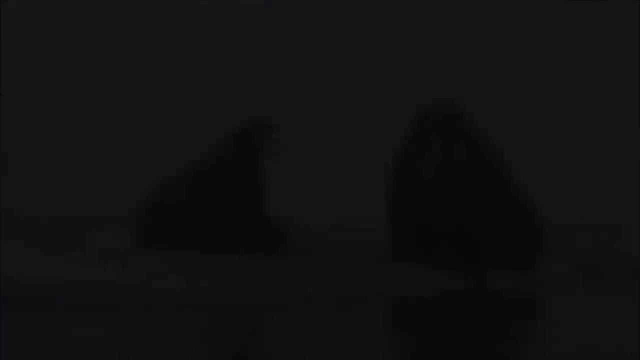 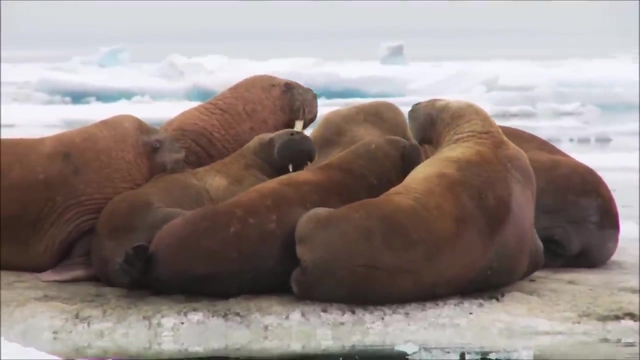 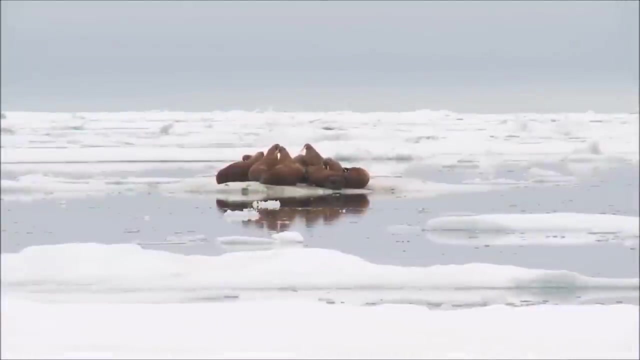 Instead, they begin in the sea. The walrus is at home on the land, in the water or on the ice. They sleep and rest on beaches or on ice shelves. They prefer to live near shallow waters. Walrus cannot dive as deeply as their relatives, the harp seals, and must be able to reach 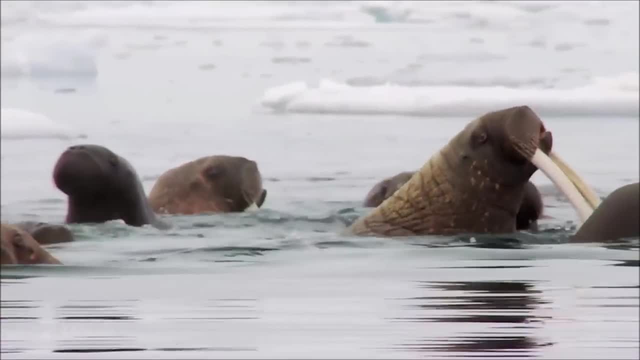 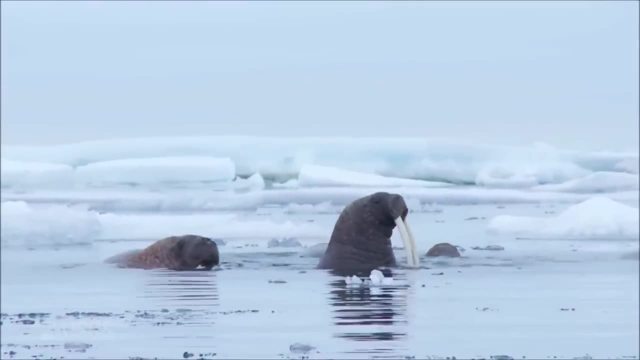 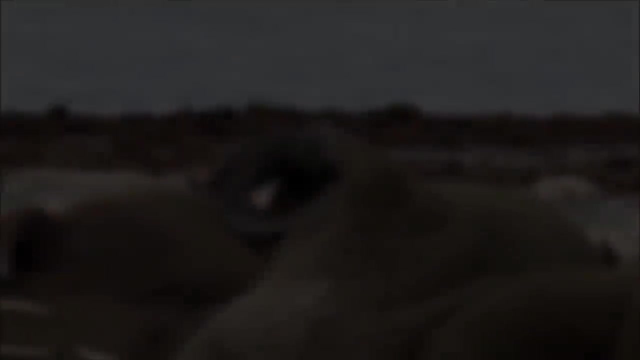 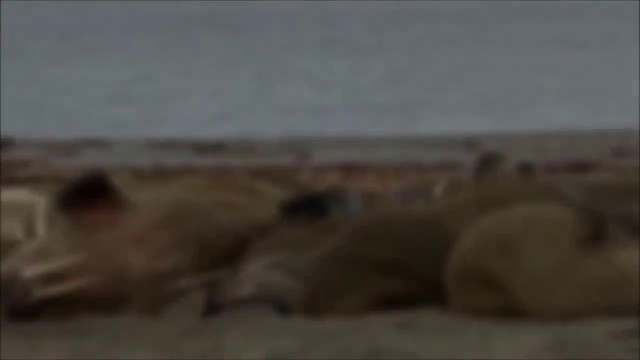 the sea floor to find their favorite foods: Clams, Mollusks And oysters. They may look peculiar, but walruses are well adapted to their icy habitat. Their wrinkled skin is nearly 4 inches, or 10 centimeters, thick in places, and the layer 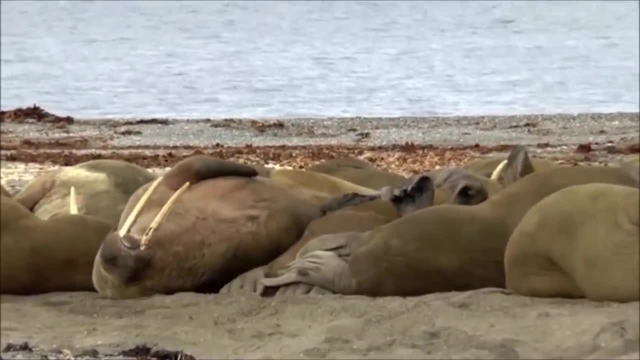 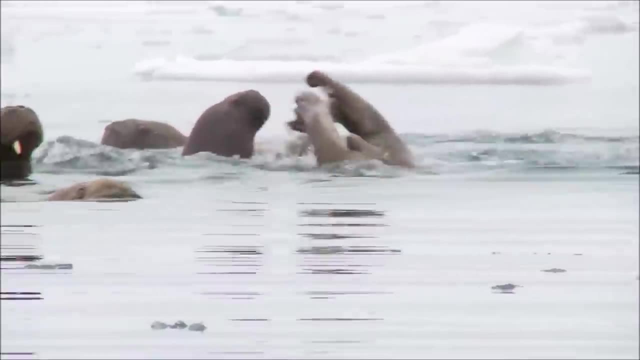 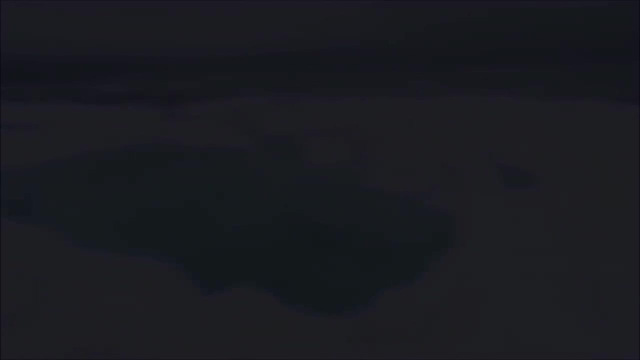 of fatty blubber beneath it is even thicker – nearly 6 inches or 15 centimeters. The purpose of both is the same – to allow walruses to stay warm in freezing Arctic waters. Thick skin and thick blubber contribute to the walrus's massive size. 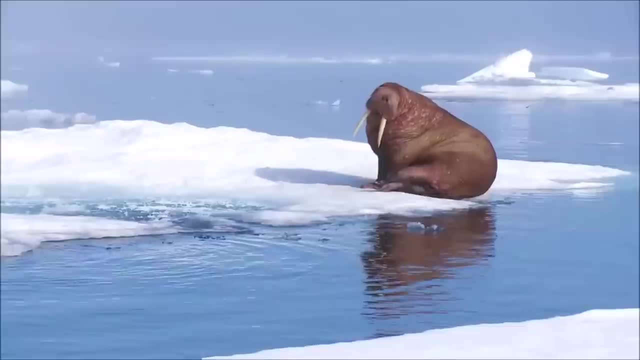 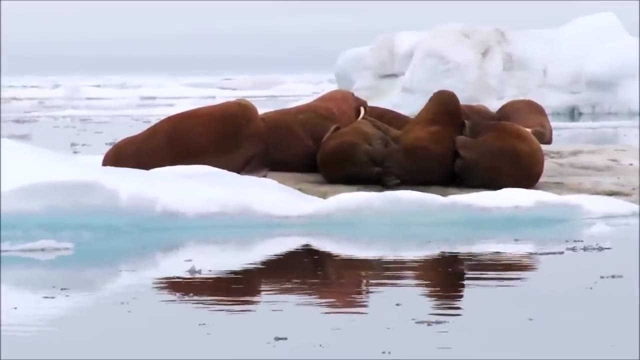 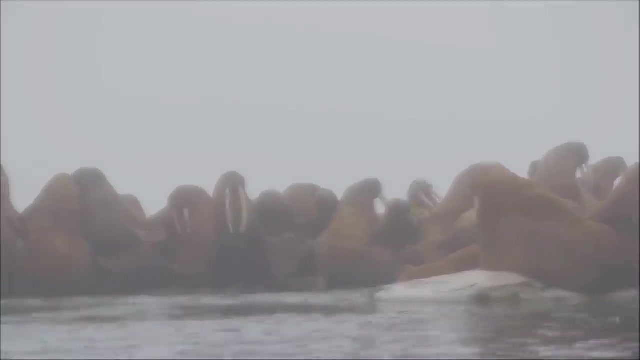 Adult males often weigh more than 2,000 pounds or 900 kilograms, and some even weigh double that. And then there is the white-winged, The black-winged. They are very strong By far. their most recognizable trait, however, is their tusks. 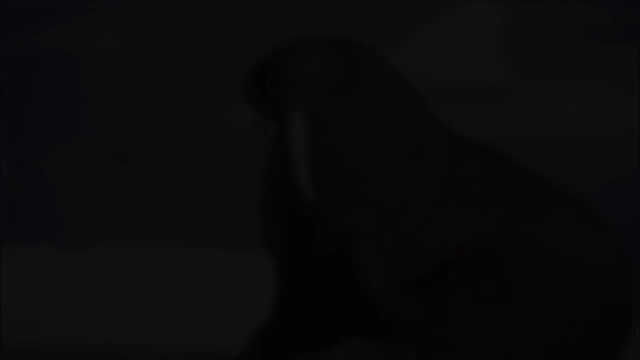 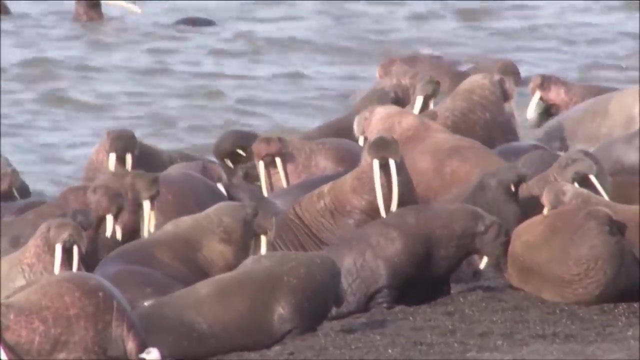 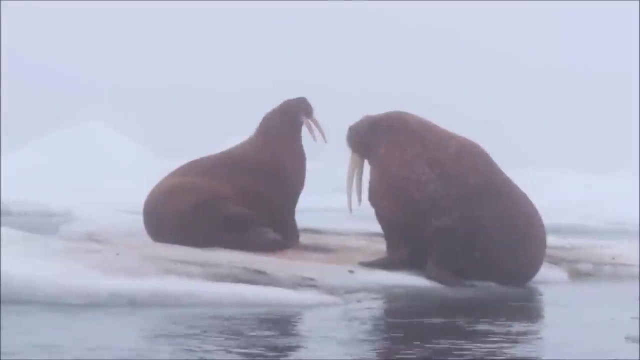 Both male and female walruses grow tusks. Tusks are in large teeth that can grow about three feet or a meter in length. Walruses use their tusks like ice picks to help pull themselves out of the water onto sheets of ice. 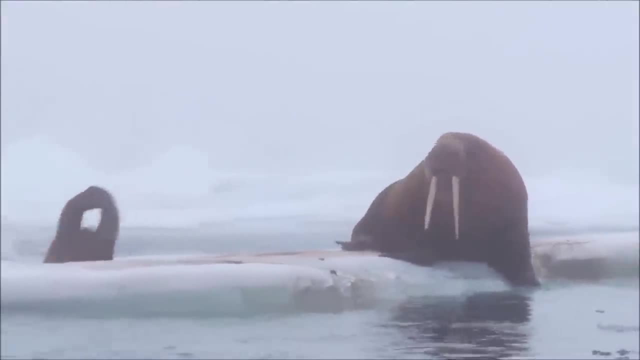 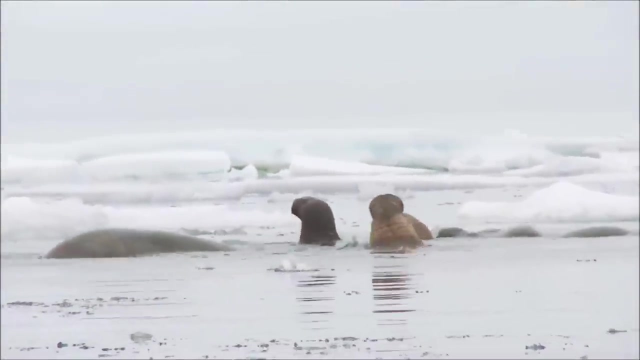 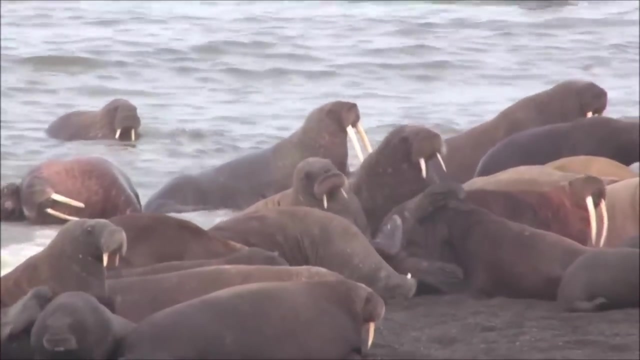 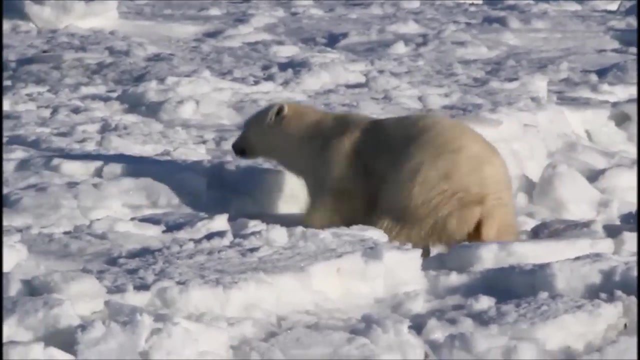 They also use their tusks to clear breathing holes when ice covers too much of the water's surface. Finally, tusks provide some defense against the only animals that prey on walruses – killer whales and polar bears Because of their harsh Arctic habitat. 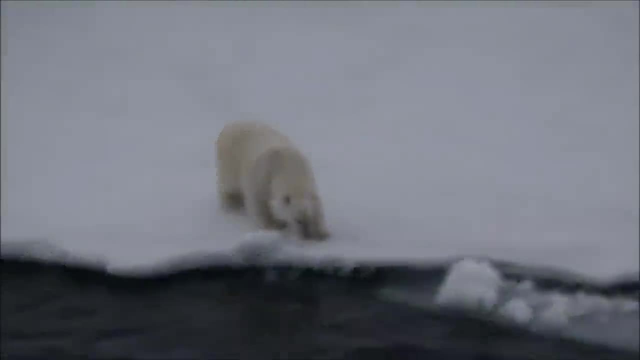 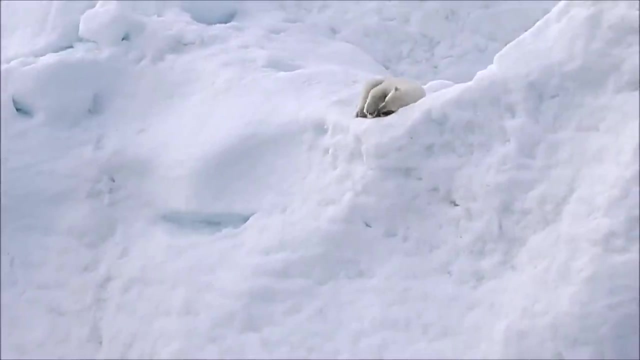 polar bears rely more on their tusks than on their females. Polar bears rely more on their tusks than on their females. Polar bears rely more on meat than any other bear. They eat mostly seals waiting at breathing holes in the ice for them to pop their noses. 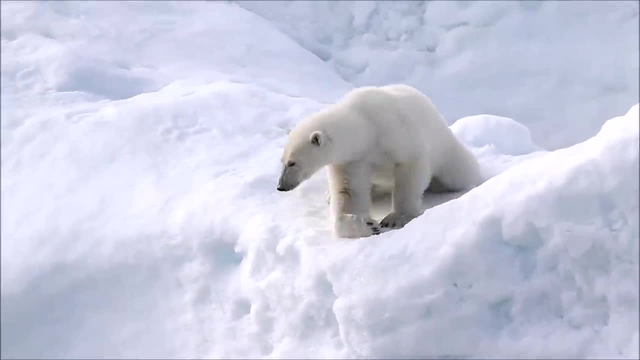 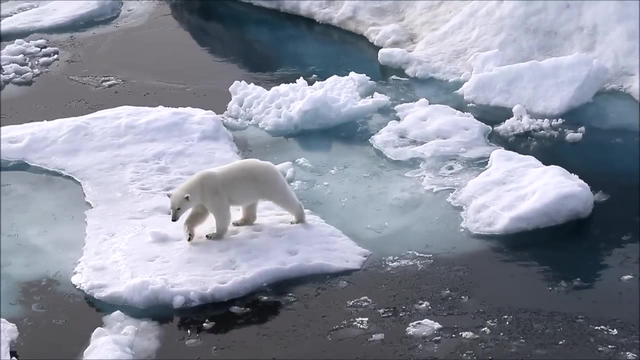 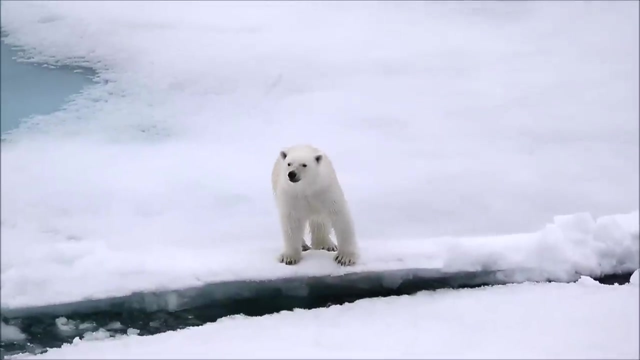 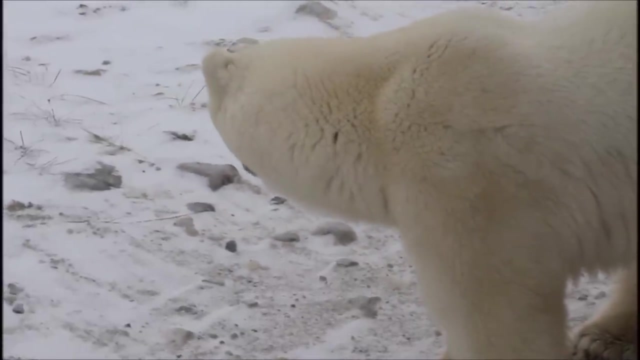 through the surface of the water and then dragging them up onto the ice. Sometimes they will catch beluga, narwhal or young walruses this way, but larger prey of this kind is much more difficult to manage. Polar bears are the largest land predators in the world. 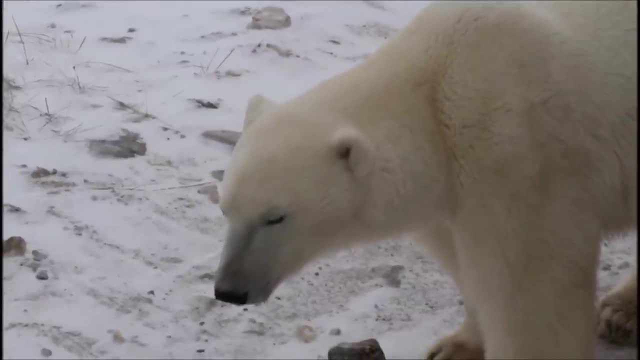 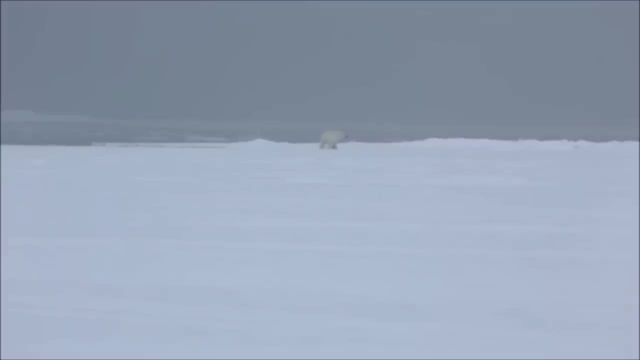 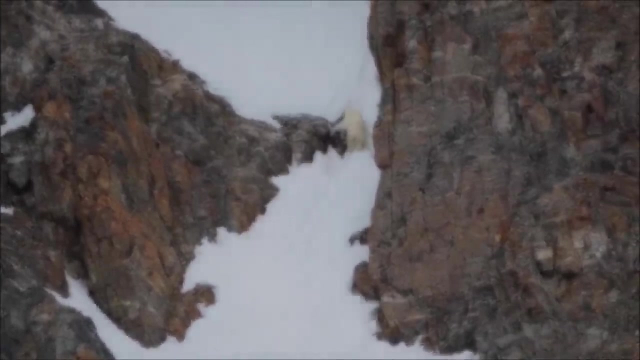 But they are also excellent swimmers, sometimes swimming for days at a time to move between hunting grounds. Like the walrus, polar bears are well adapted to their harsh Arctic habitat. Thick white fur serves as camouflage as well as insulation. Polar bears are the largest land predators in the world, but they are also excellent. 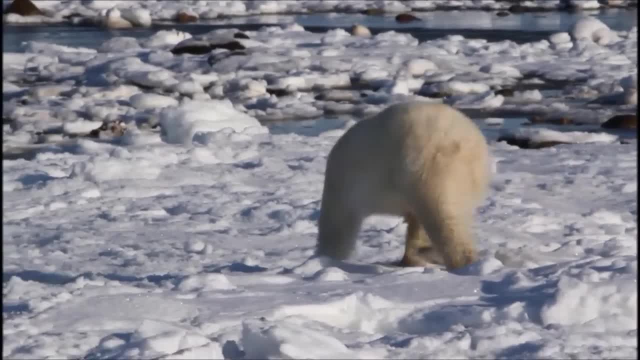 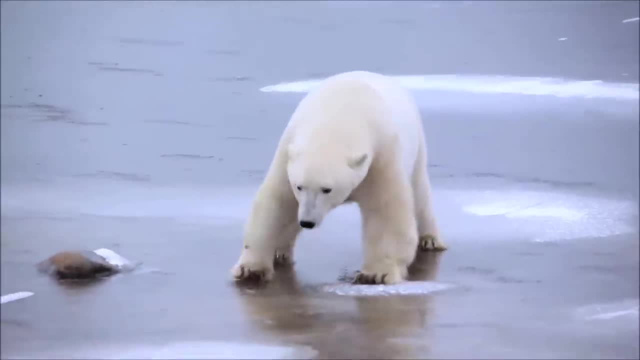 swimmers, sometimes swimming for days at a time, to move between hunting grounds And a layer of blubber underneath provides extra warmth. Their paws are extra wide to help them distribute their weight and allow them to walk on top of snow or thin ice without breaking through. 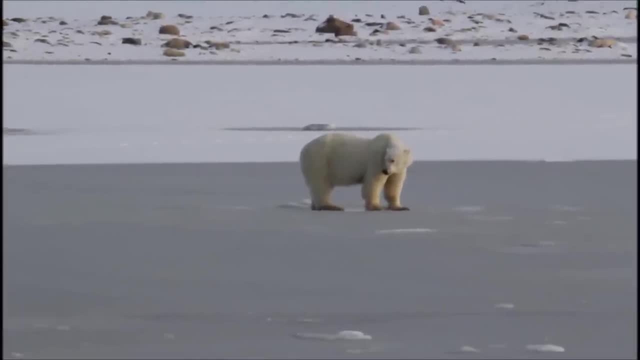 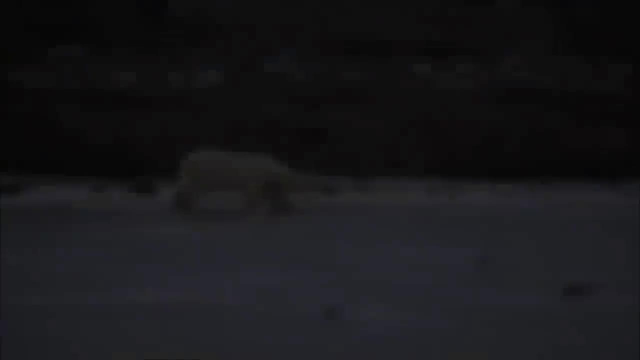 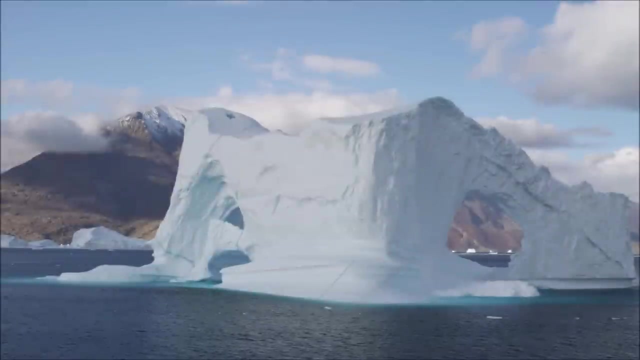 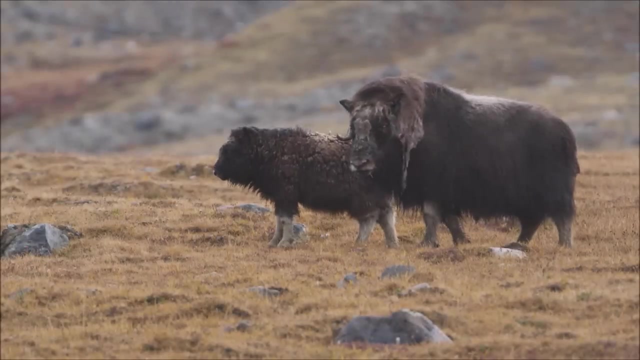 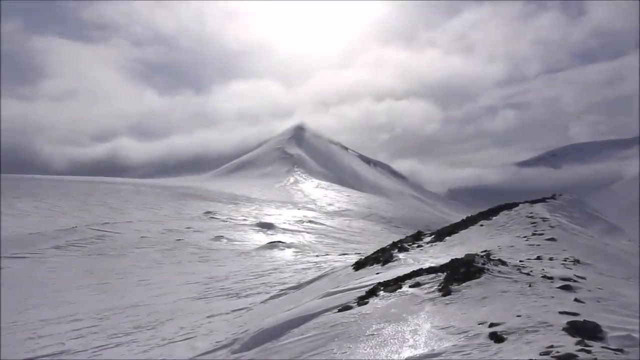 And their thick, strong claws help polar bears grab onto slippery prey as well as better grip the slippery ice. The Arctic is a harsh, forbidding land, but it is far from lifeless. Plants and animals live and grow and flourish in the conditions they are adapted for. 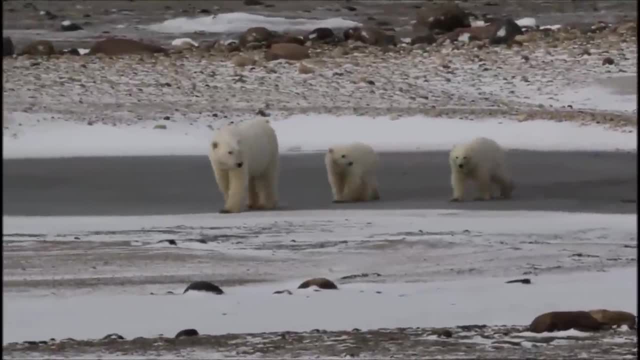 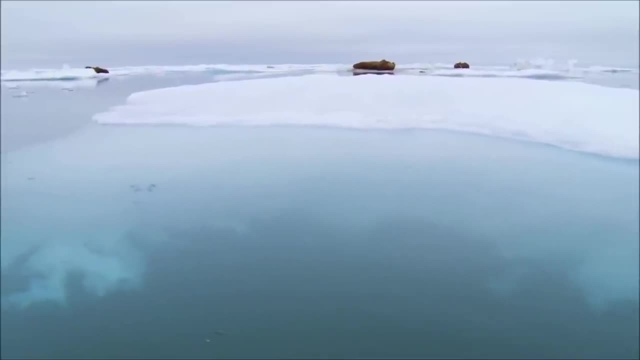 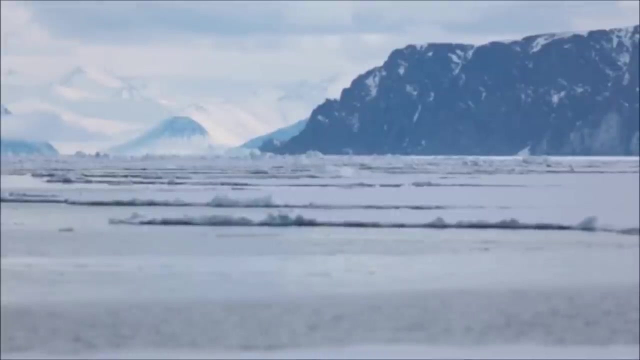 Many species depend on the cold and the ice and would not be able to survive if it was gone, Because the arctic climate is so unwelcoming to humans. much of it has gone, untouched and undeveloped, but we can still disturb the delicate balance these creatures depend on. 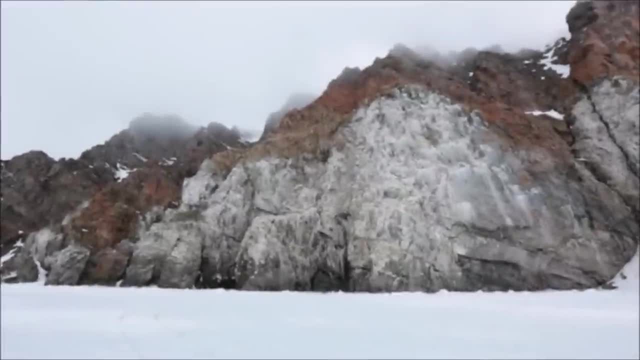 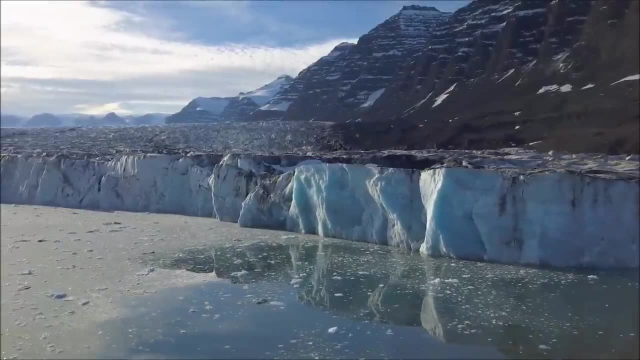 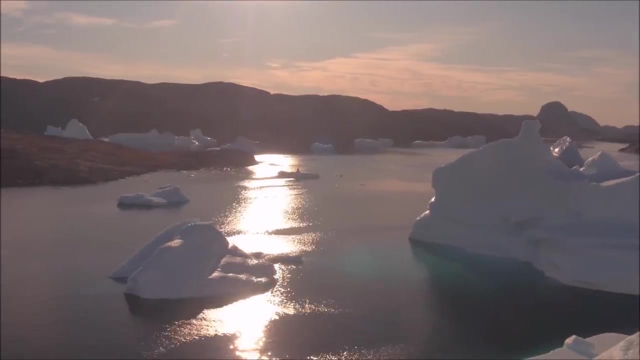 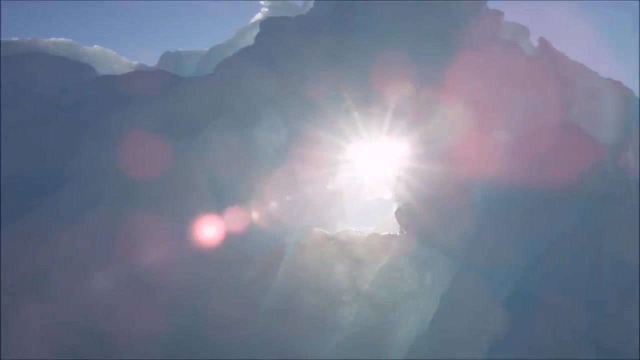 Hunting, pollution and gathering natural resources may cause changes that upset the network supporting life in the northernmost reaches of our planet. I hope you learned a lot today about the arctic, the land of the midnight sun. Goodbye, till next time. 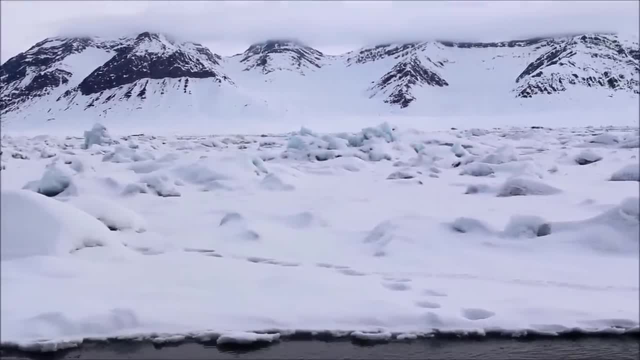 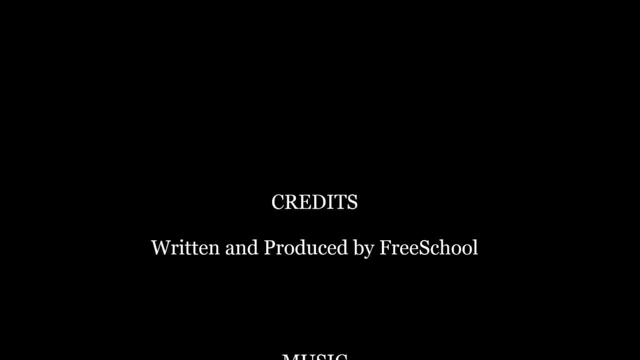 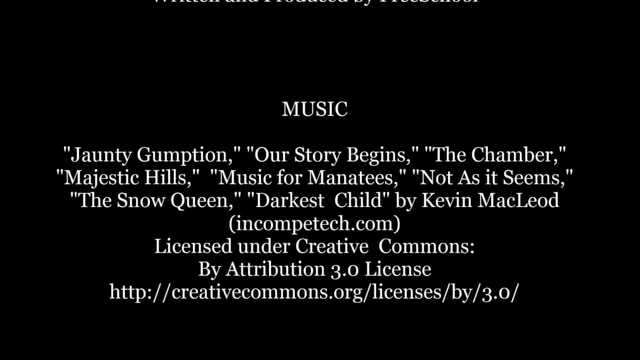 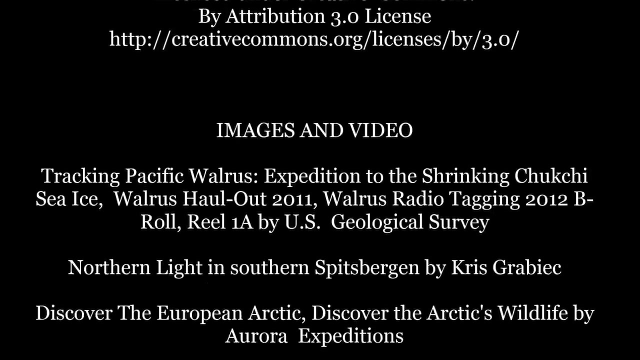 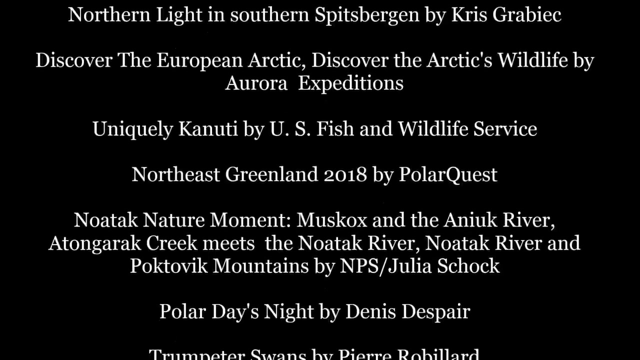 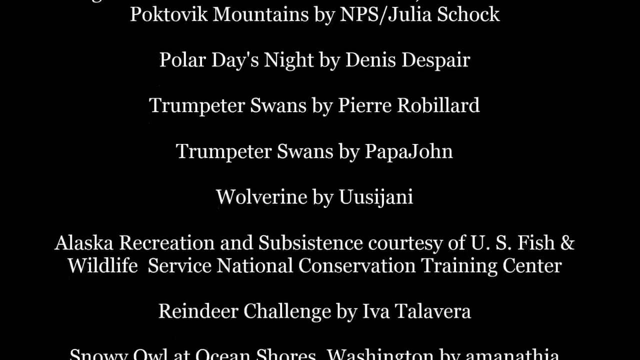 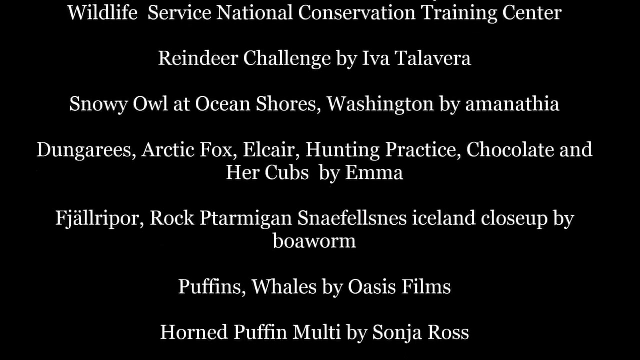 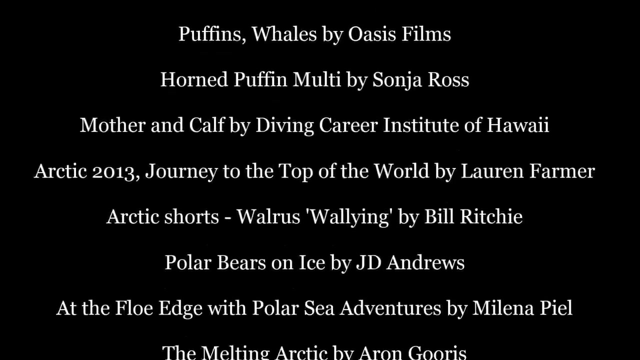 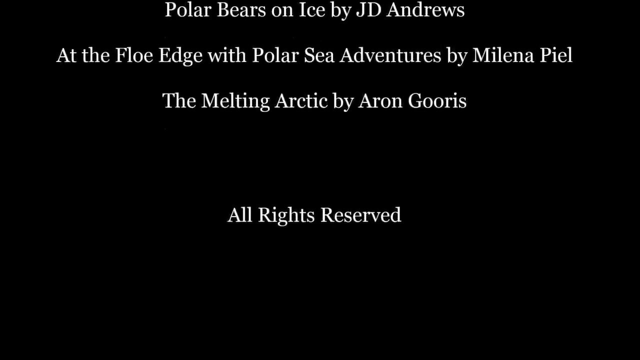 Thank you for watching. I hope you learned a lot today about the arctic, the land of the midnight sun. Good luck. Thank you for watching.